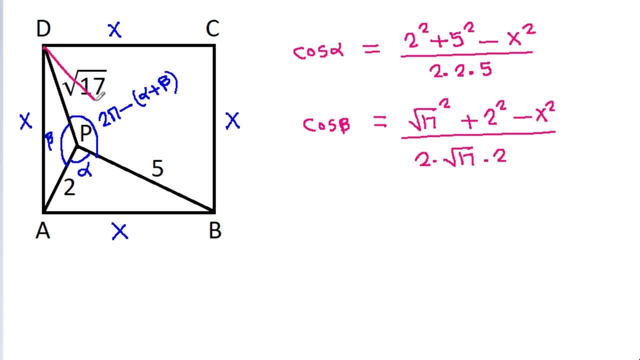 And if we join DB then this angle is 90 degree, So diagonal of a square it will be root 2 x. So in triangle BDP cos 2 pi minus alpha plus beta it will be equal to root 17 square plus 5 square minus root 2 x square by 2 times root, 17 times 5.. 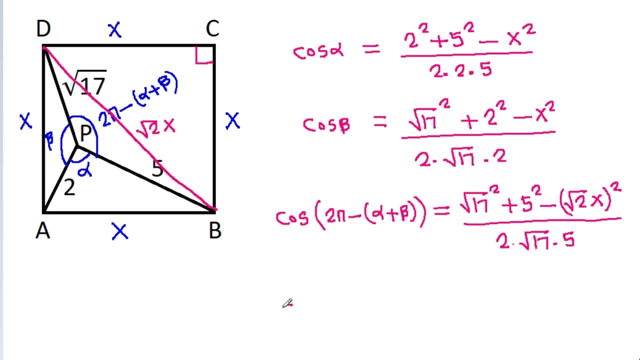 And cos 2 pi minus alpha plus beta will be cos alpha plus beta is equal to 17 plus 25 minus 2 x square by 2 times root, 17 times 5.. And cos alpha plus beta, it is equal to cos alpha, cos beta minus sin, alpha, sin beta, And we have cos alpha, cos beta. and from here 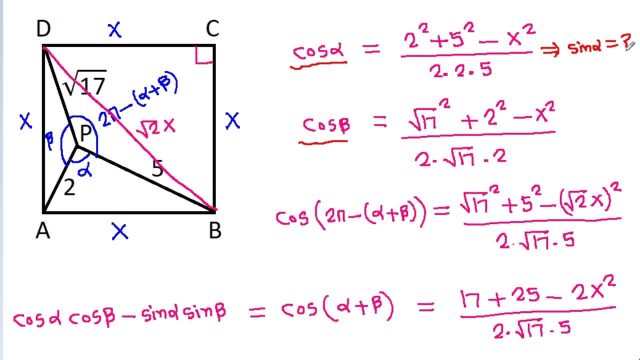 I will write sin beta, and I will write cos alpha, cos beta, and from here I will write: we can find sin and from here we can find sin, and then we can put the value of cos, cos, sin and sin and we can find the value of x square. But this will be very lengthy process. 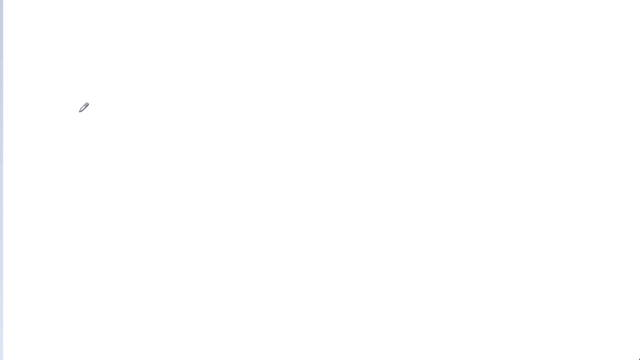 So I will solve it by second method. This is the square and the length is 2, 5, and root 17.. And if we add root 17 square and 2 square, then it is not equal to 5 square. 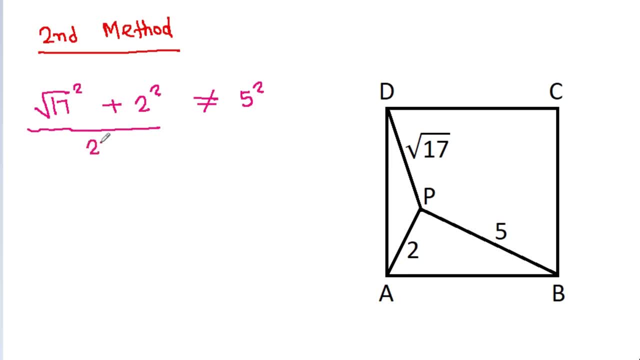 Because this is 17 plus 4, 21, and this is 25.. But 17 plus 8, it is 25.. That means root 17, square plus 2, root 2, a square is equal to 5a square. 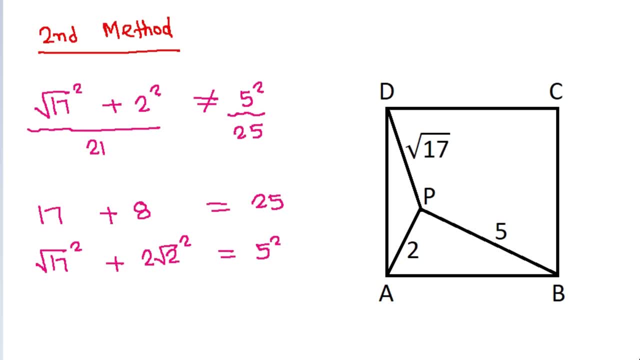 And we have root 17.. So if we draw a perpendicular from A of length 2, and join these two points, then this length will be 2 root 2.. And if this length is 5,, if it is 5,, 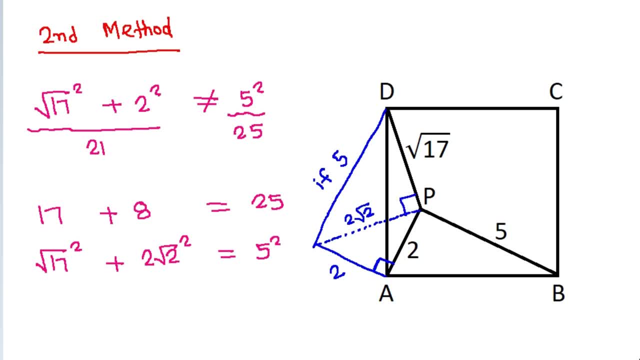 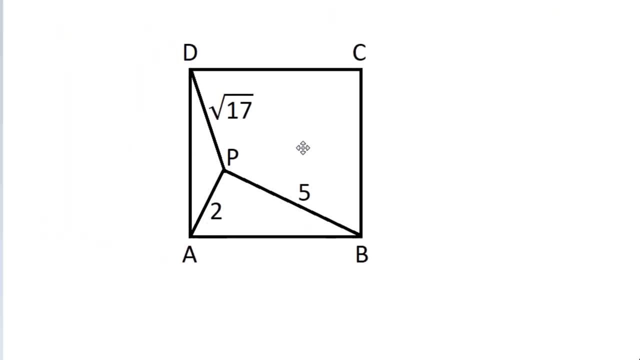 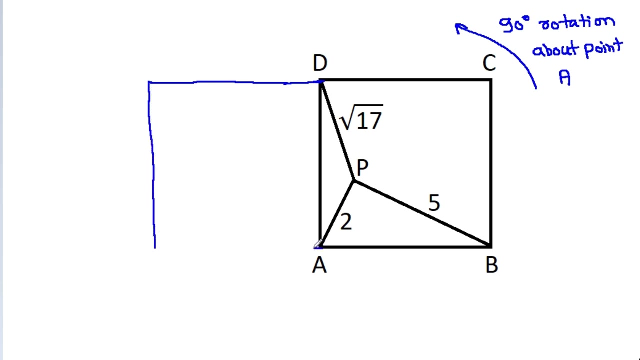 then this angle will be 90 degree. So this is the square, And if we rotate this about point A by 90 degree- 90 degree rotation about point A- then this point will be D dash And C will come here, C dash. 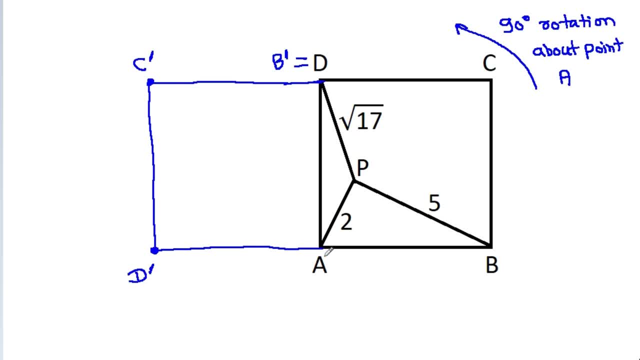 And B dash and D will be same point And A and A dash is same point And P will come here. suppose P dash And this angle will be 90 degree, Because we are rotating by 90 degree And AP is 2.. 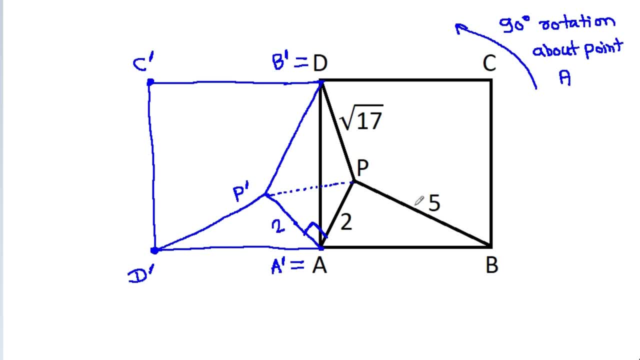 So A dash P dash will be 2. And BP is 5.. So B dash P dash will be 5. And DP is root 17.. So D dash P dash will be root 17. And this length will be 2 root 2.. 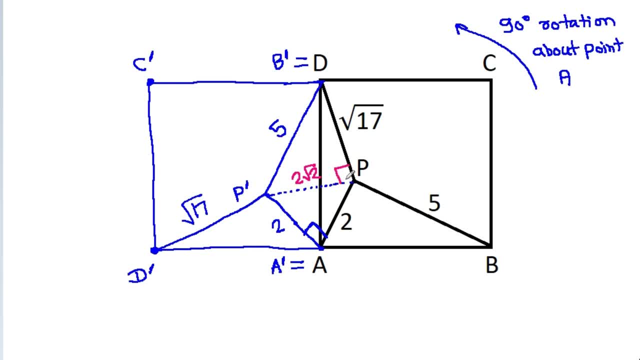 And this length is 5.. So this angle will be 90 degree And also inter angle AP, P dash. AP dash is equal to AP, So these 2 angles will be equal to 45 degree. So angle AP D is equal to 45 degree plus 90 degree. 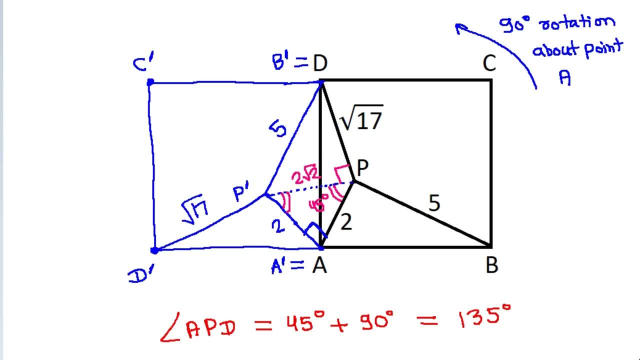 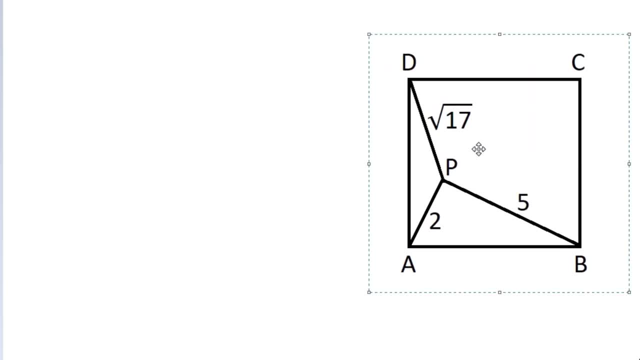 That is 135 degree. So this is the square And this angle theta. it is equal to 135 degree And side length of a square is x. So now we can use cosine root inter angle ADP. inter angle ADP. 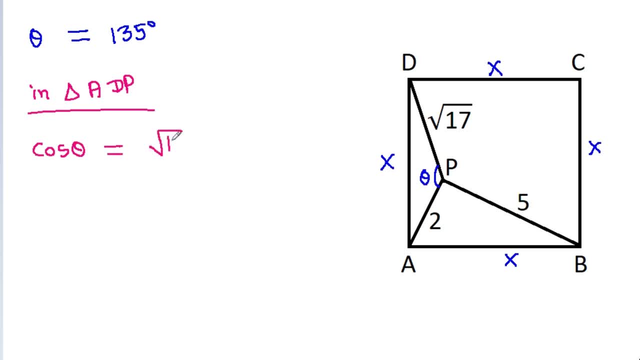 cos theta will be equal to square root of 17 square plus 2 square minus x square by 2 times square root of 17 times 2.. And it is, cos theta is 135 degree, is equal to 17 plus 4 minus x square. 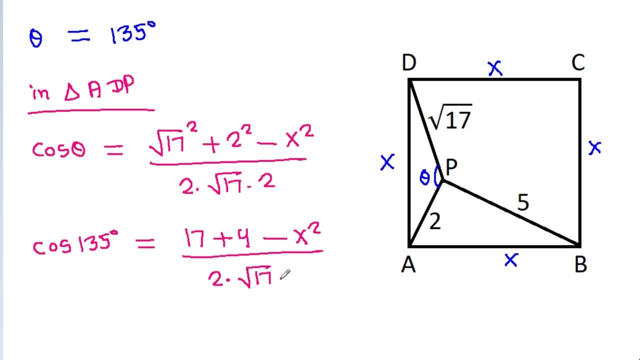 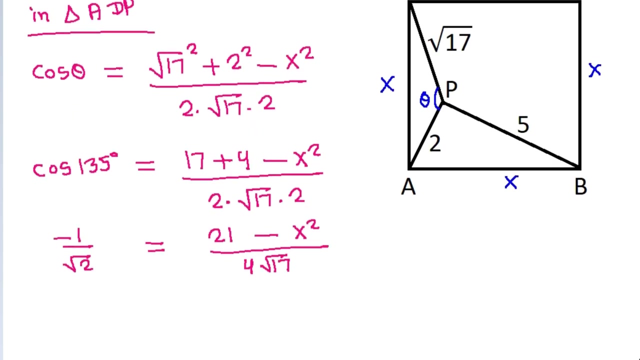 by 2 times square root of 17 times 2.. And cos 135 degree is minus 1 by root 2 is equal to 17 plus 4, is 21 minus x, square by 4 root 17.. And it is minus 4.